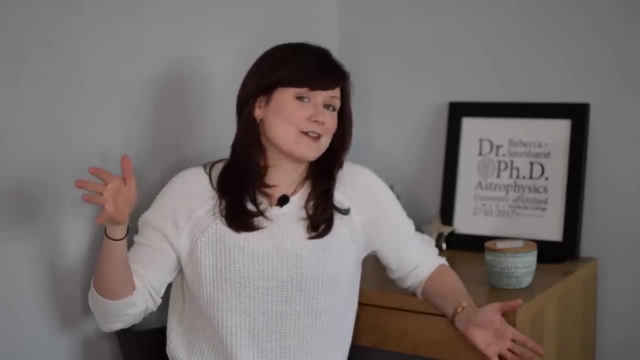 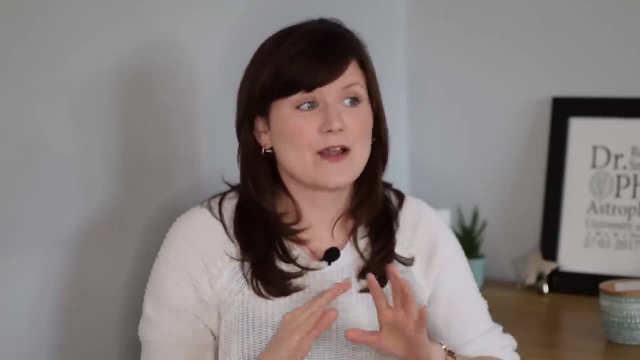 further, So I didn't feel like it was something that I could leave out. And finally, just before I get into this, I want to acknowledge that my path comes from a place of great privilege. I was very lucky to be born in a country where girls education is a given. It's not questioned. I was very lucky. 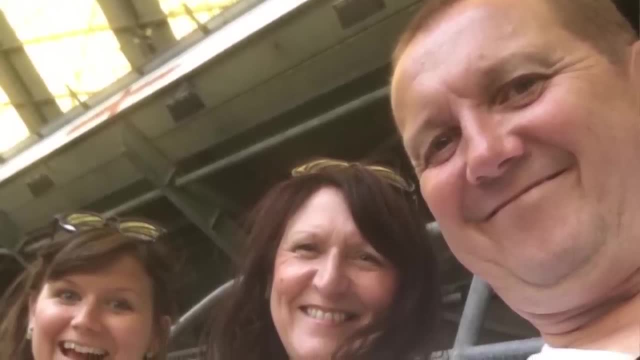 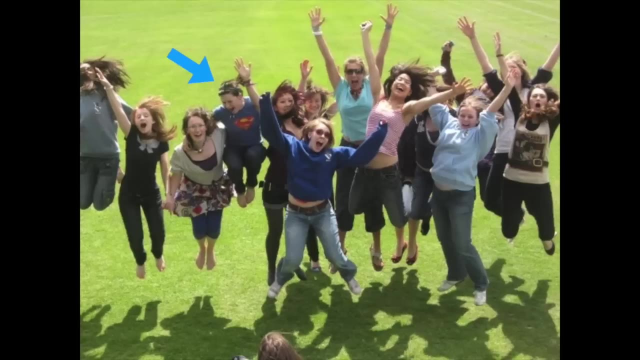 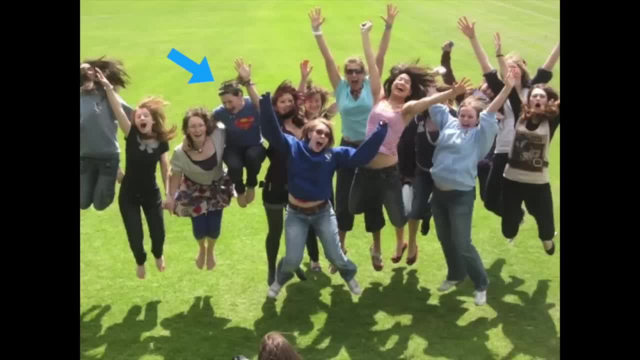 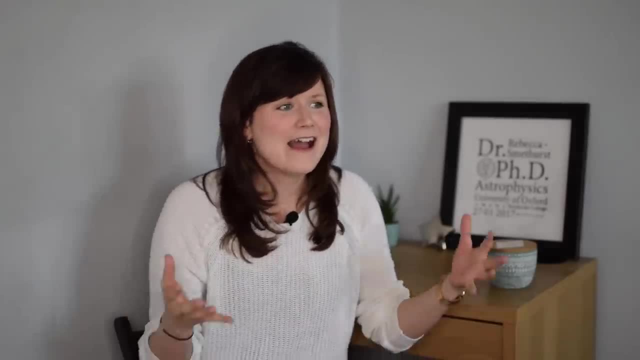 societal norms that say that there are subjects that girls do and girls don't do, which is the stupidest thing I've ever heard. Please don't ever tell any kid that I just went to a school where there was the subjects the cool kids did and there was the subject the cool kids didn't do. 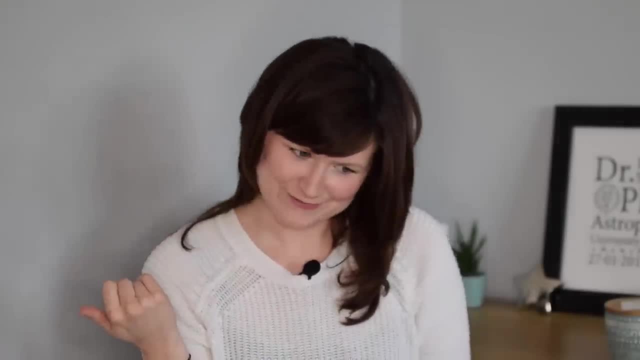 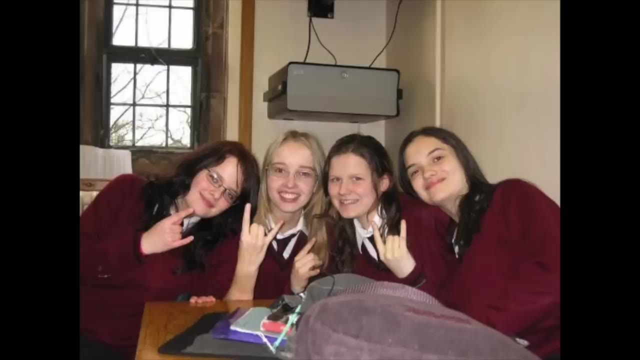 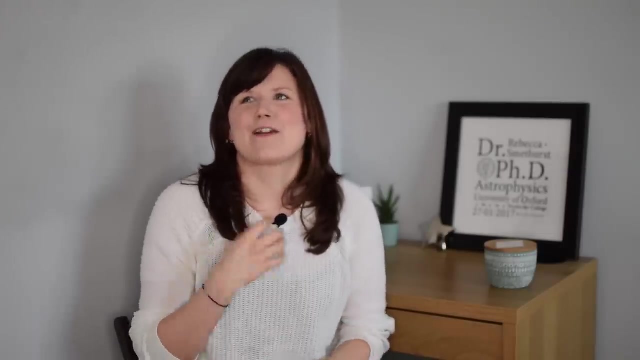 And obviously the cool kids did physics, Obviously. So I want to start when I was 14 years old in high school- This was year 10 in the UK and physics was my least favourite subject, Surprisingly. I even remember vividly, like my French oral for my GCSE being like: 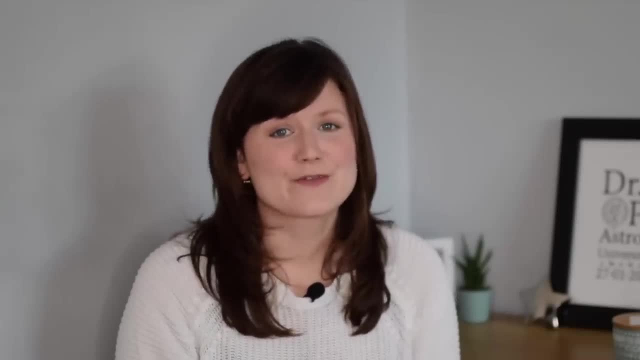 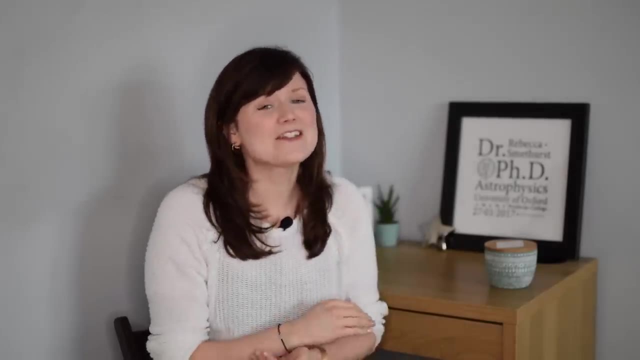 J'adore l'histoire, mais je déteste la physique. I had a very high-pitched voice in school, But, luckily for me, science was a compulsory subject for all people in the UK taking GCSEs, And so that by the time I was 16, physics had actually become 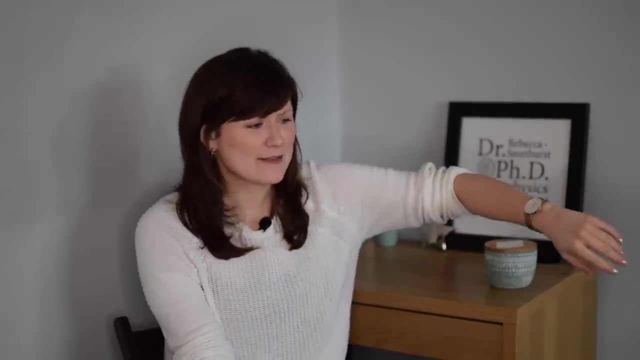 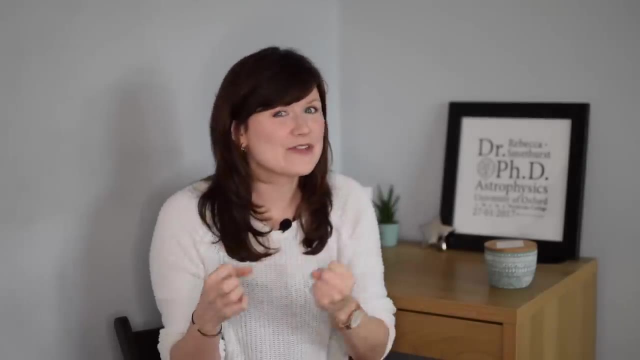 my favourite subject because we'd stopped doing all the stuff that we were doing in the lower years on, like forces and light travels in straight lines, And we'd started doing really cool stuff like radioactivity and astronomy- And astronomy was something that I had loved since I was a kid. I was obsessed. 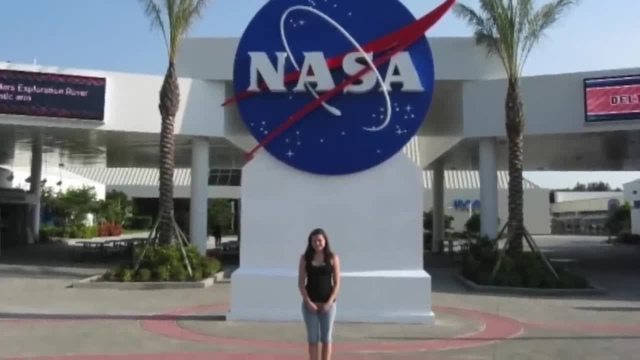 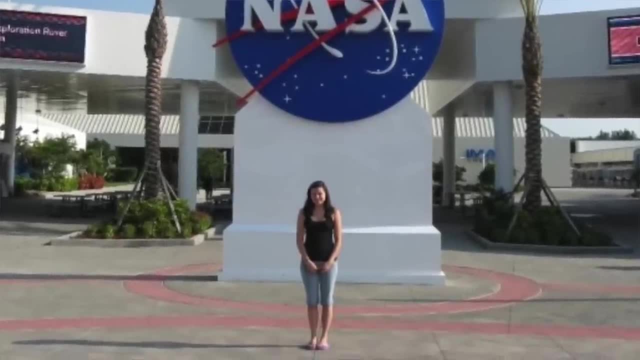 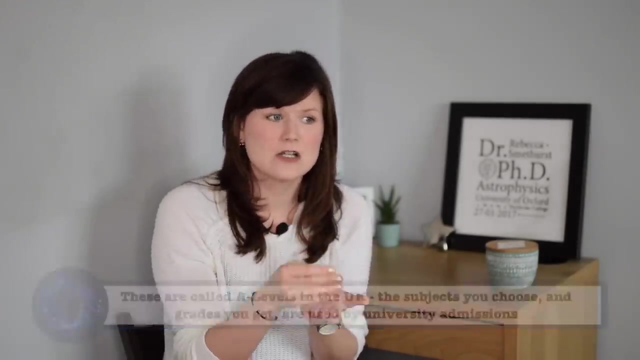 with space, And it was at that point I realised that actually space is physics, And so if I wanted to learn more about it, I'd need to take physics. So when I was 16 and it came to picking the four subjects that I would take further into my final two years of high school, So I chose maths. 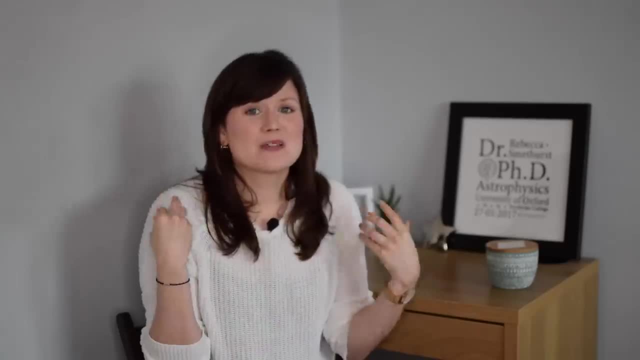 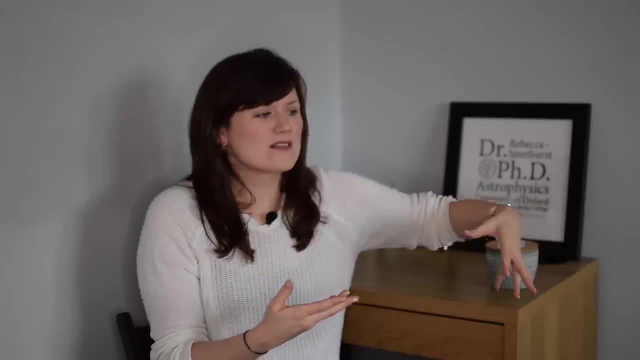 further maths, physics and chemistry, But I chose them because they were my favourite subjects At the end of the day. when I'd come back with a huge pile of homework at home, they were always the ones that I would pick off of the pile first to be like: well, let's get the 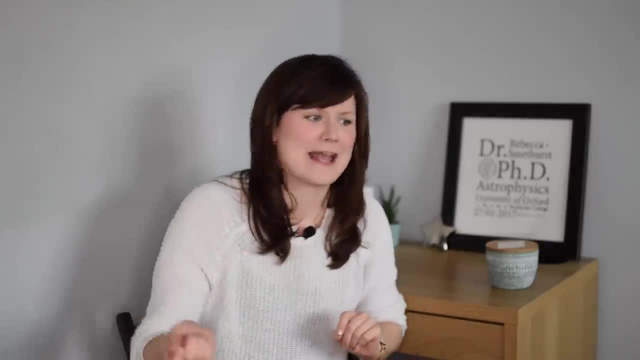 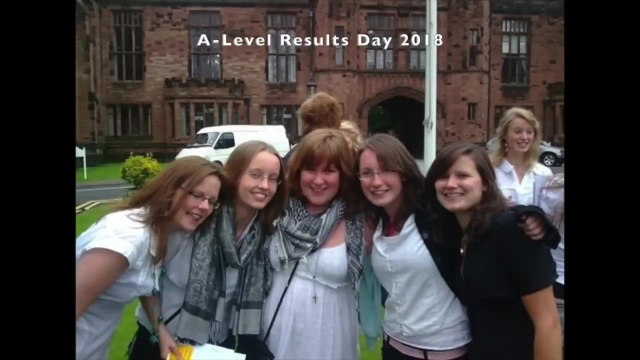 maths homework done first, because I can do that and I get it and we'll deal with that massive English essay later. I ended up getting all A's in my final exams for my A levels, which I am still immensely proud of to this day Now. good grades aren't everything to travelling the path to being a scientist Like. for me, they were literally just a hoop to travel the path to being a scientist, But I'd done it and I was still extremely proud of it. So there were some good grades I had, But I'd also got a lot of A's in my final exams that I was proud of. So I'd still get a lot of A's in my final exams. 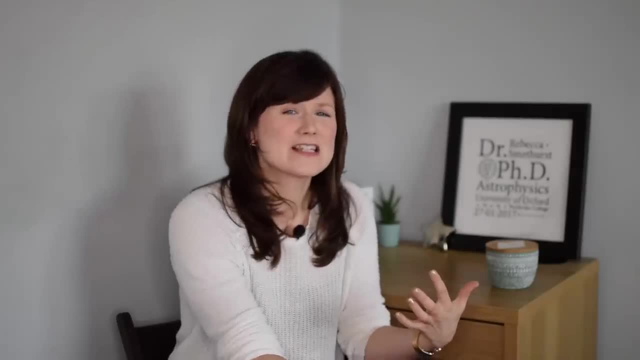 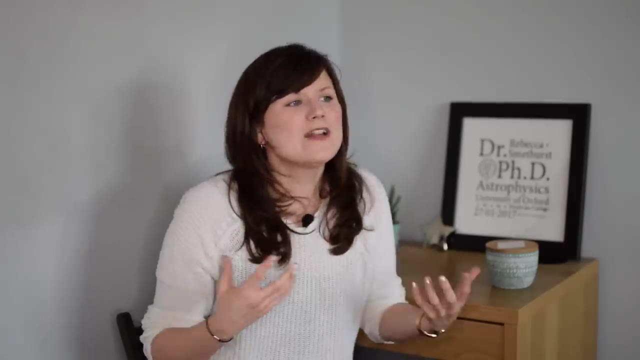 just a hoop to jump through in order to get into university, but you'll find that good grades do open more doors for you. So just remember: practice makes perfect. You wouldn't expect to pick up a violin and be amazing at it the first time round. You can't immediately become fluent in a language. 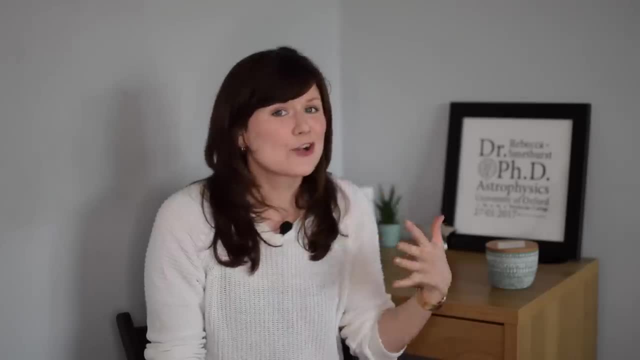 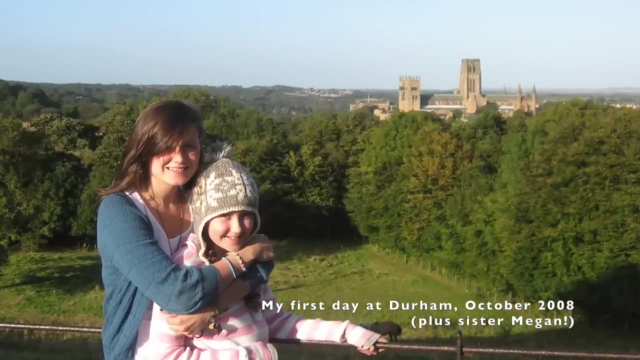 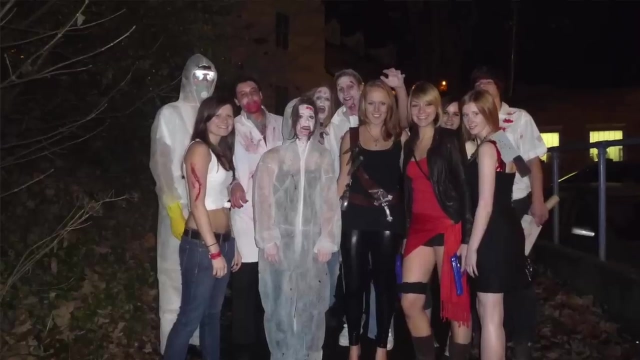 overnight. It's the same for maths and science. You really got to work at it until it becomes second nature to you. But those grades meant that I got into Durham University to study physics with astronomy when I was 18.. I loved my time at university. I went to Aiden's College at Durham. I 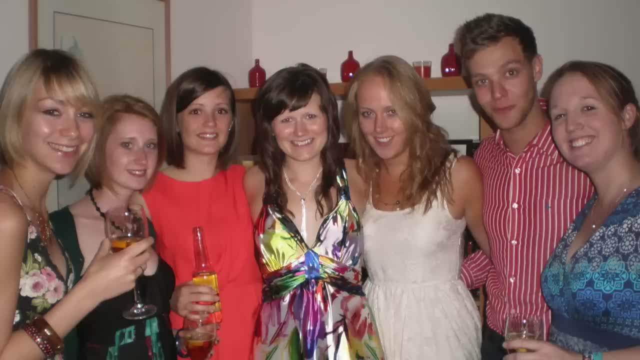 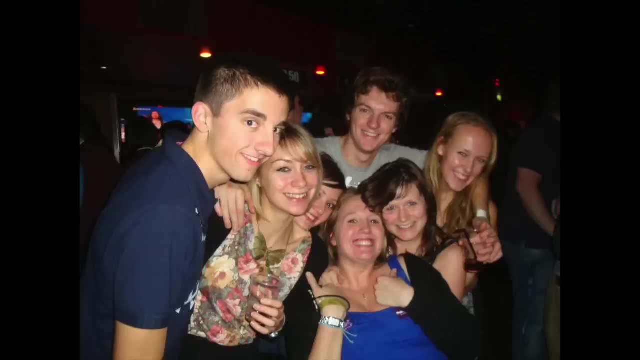 met some absolutely wonderful people and lifelong friends. I got to use the telescopes on top of the roof of the physics department, which was awesome and also had some incredible nights out while I was there as well. I was there for four years because I did what's called an undergraduate. 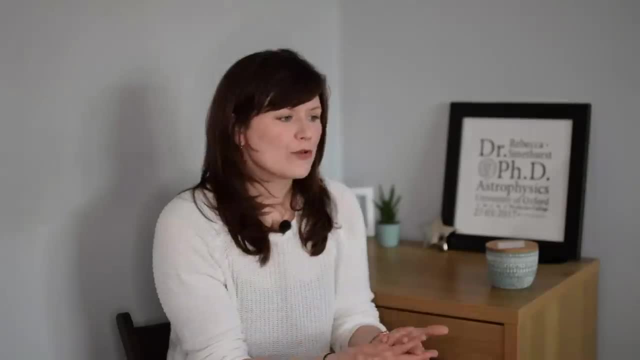 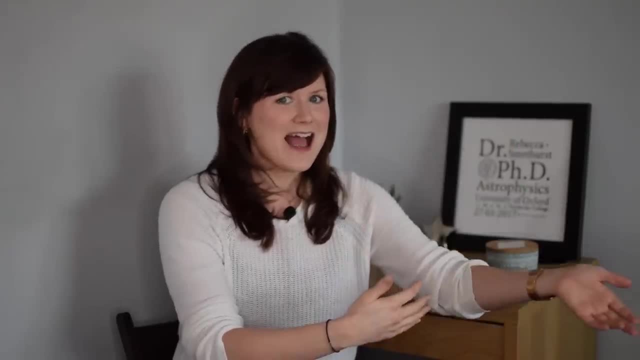 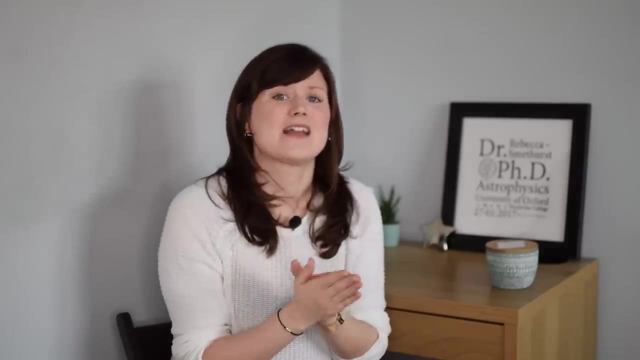 bachelor's of science and then you graduate and then you go on to do your master's. I did my master's all the while without graduating, So my friends might have graduated after three years. I didn't graduate until four years, So my first three years were essentially just being taught. 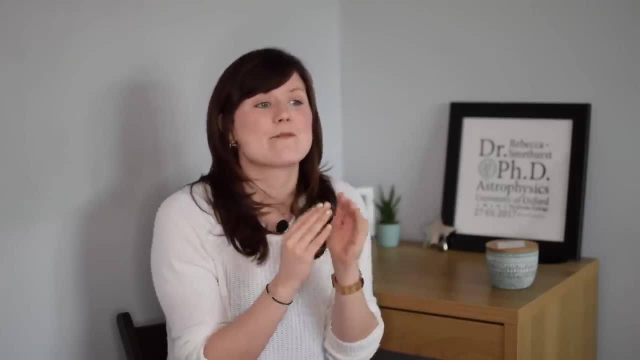 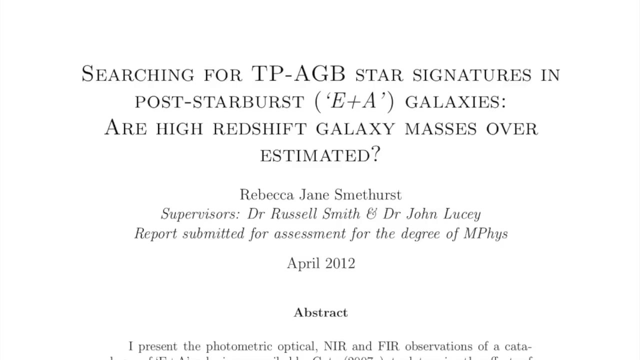 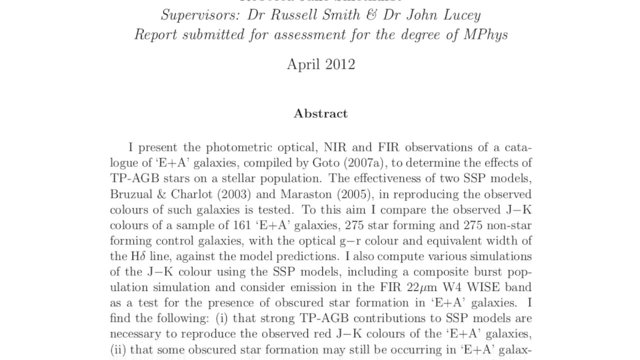 lots of lectures, a couple of different like lab projects, and then in my fourth year it was all about research. Half of my entire mark for the year was going to be the research project that I was doing with a project supervisor who was a sort of a professor or a researcher in the department, who was basically advising, like 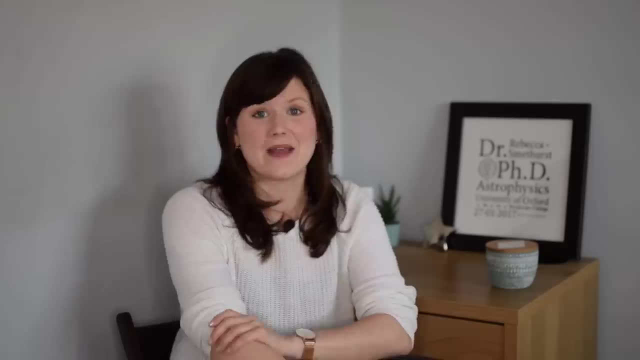 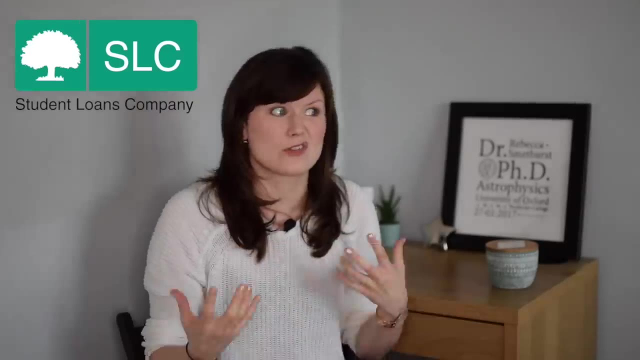 what science we would do and what questions we were asking. Now I didn't pay for my university course. I took a student loan, which is very commonplace in the UK. There's this massive central system that's all done through the government. It was about £3,225, I think, per. year in tuition and then £3,000 a year as a living cost loan. So every year I was essentially borrowing just over £6,000 to go to university times. that by £4,000.. So I was basically borrowing just over £6,000 to go to university times. that by £4,000. So I was basically borrowing just over £6,000.. So I was basically. borrowing just over £6,000 to go to university times. that by £4,000.. So I was basically borrowing just over £6,000 to go to university times. that by £4,000.. So I was basically borrowing just over £6,000.. So I ended up with. probably about a £25,000 loan. Okay, that's a lot of money. The whole idea is that you do not start paying it back until you start earning, and it comes straight off your wage as well, So it's almost like you don't. miss it because you never see it before you pay it back. Also, you pay it off in proportion to how much you're earning and it's sort of exponential. so the more you earn, the more you will pay off. But if you haven't paid it off after 25 years since you started earning, then it kind of gets. written off by the government anyway. Of course, since I went to university, UK tuition fees have actually increased from just over £3,000 a year to £9,000 a year, So I understand that people thinking about going to university in the UK today are thinking about a much larger loan. 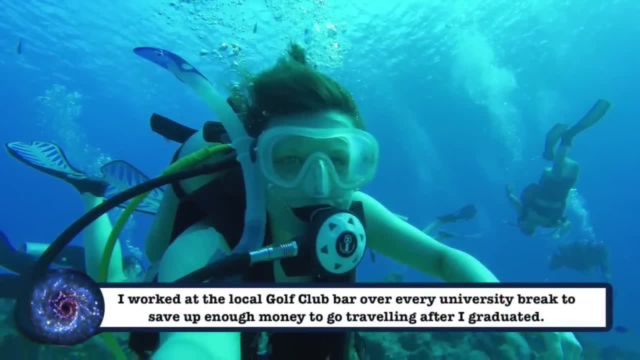 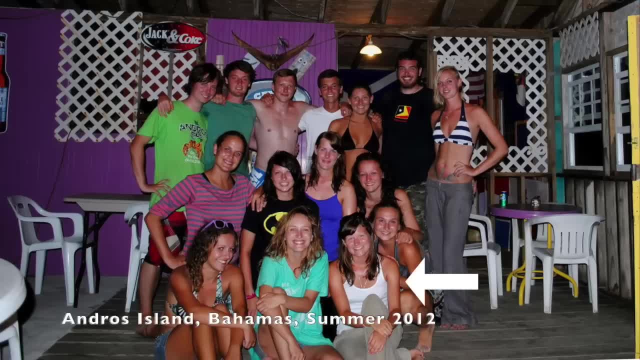 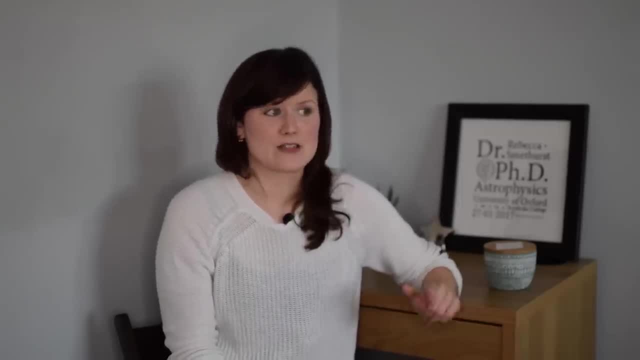 fantastic. Scuba diving is still one of my favourite things and I do it as often as I can, which is not often enough, and one of the reasons I did that was because I was terrified to leave university. I was terrified to graduate, I was terrified to find a job. 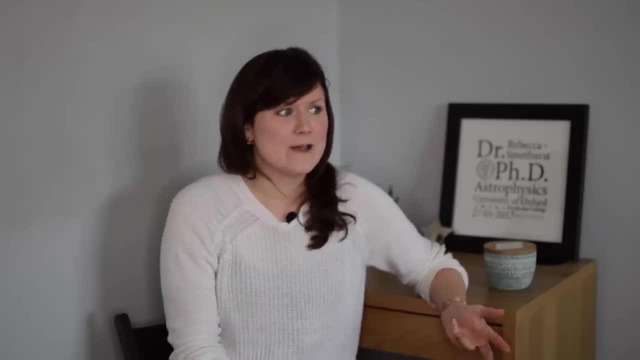 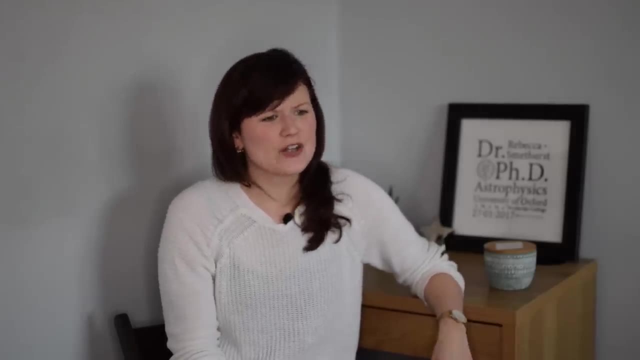 I didn't know what I wanted to do. still, I didn't really think I wanted to do research because I'd just done that research project and it was okay and it was fun. but you know, there was other things out there in the world and I was kind of putting it off for a very long time. 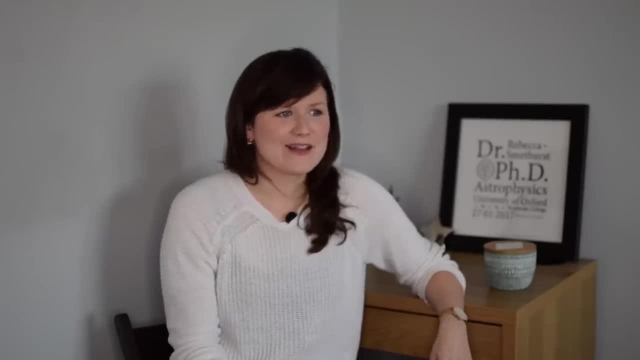 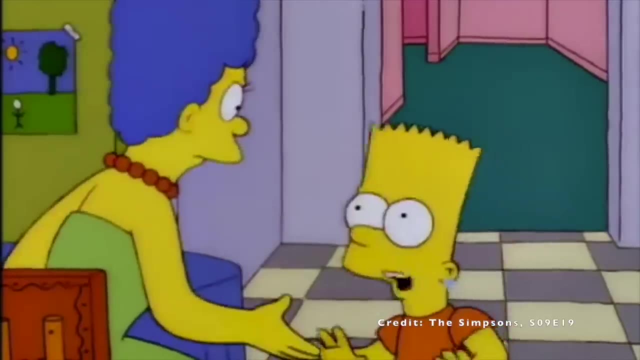 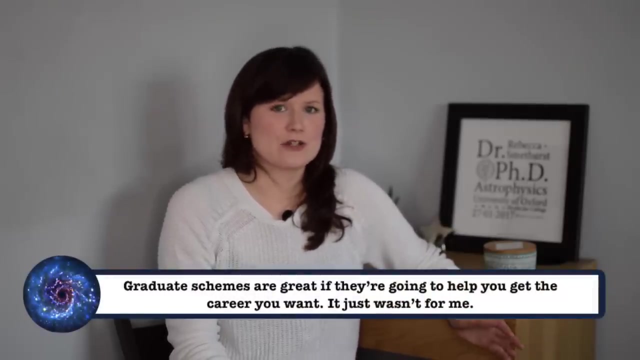 thinking about what I actually wanted to do, and so I did the classic thing that you shouldn't do, which is I did what everyone else was doing, which was applying for graduate schemes- Companies that have these big schemes to hire graduates fresh out of university and train them. 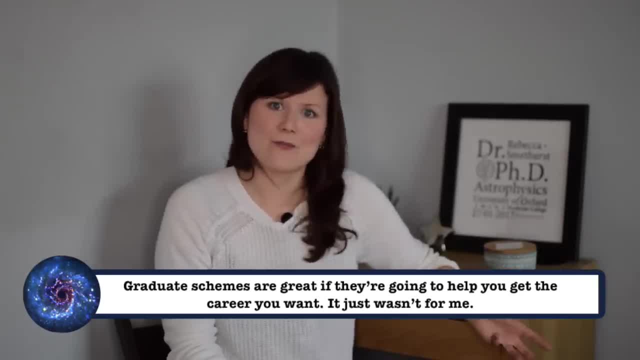 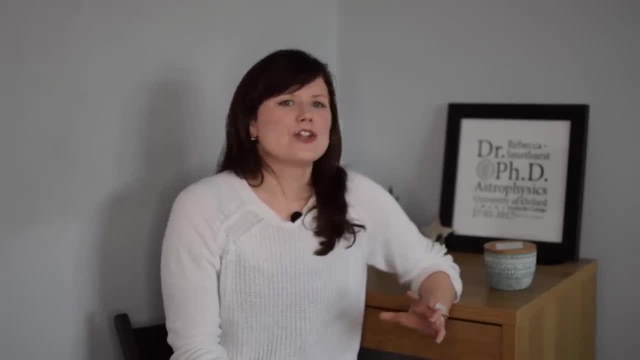 how they want to be trained so that they can progress through the company. and my idea was that I wanted to do satellite technology. I wanted to work in the space industry, you know, launch things on rockets and getting things into space, because I thought that sounded really cool. 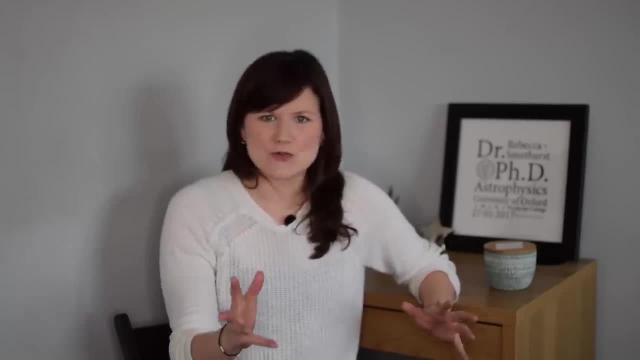 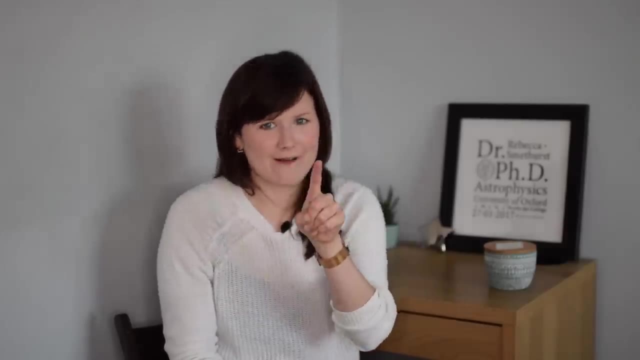 and I couldn't get a job directly with a company, say Astrium, which is the UK satellite company. I did apply for them but I didn't get the job. but I did get a job with Rolls Royce, who don't make cars, they make jet engines. and I figured jet engines rockets. they're not that far apart. 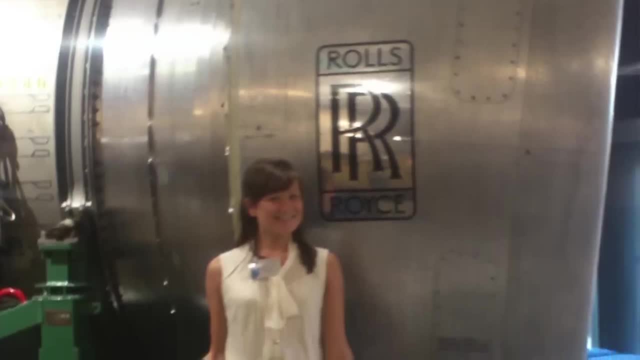 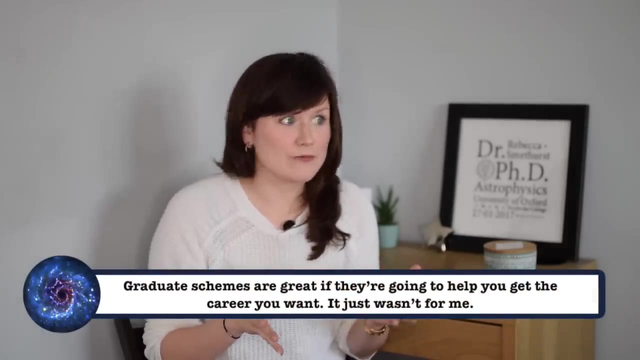 The thing is, it was an engineering grad scheme, it wasn't a physics grad scheme, it wasn't a research grad scheme either. so I realised very quickly that, even though I was doing very similar things to what I've been doing in my research project, in my masters, you know- 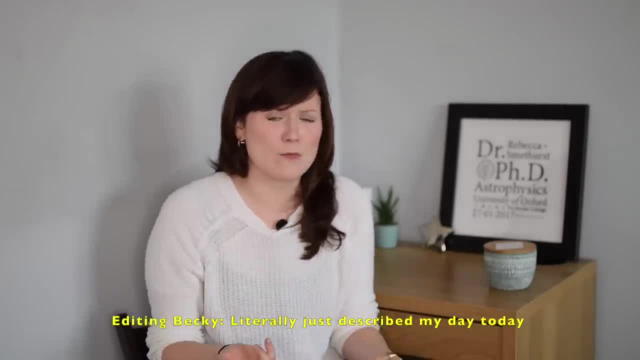 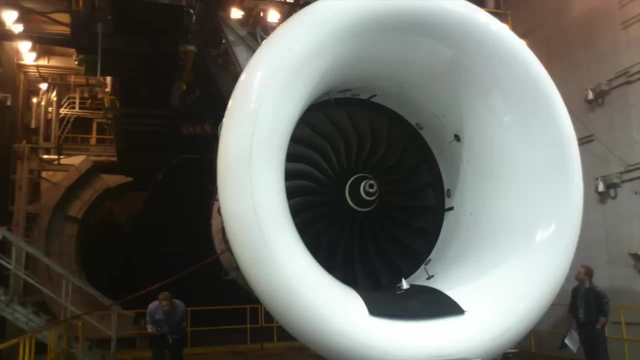 sitting crunching data, sitting at a desk all day and solving problems. I wasn't doing it for any reason that I cared about. I didn't care about the engineering things we were talking about, like test beds for jet engines and stuff. so every meeting to me was: 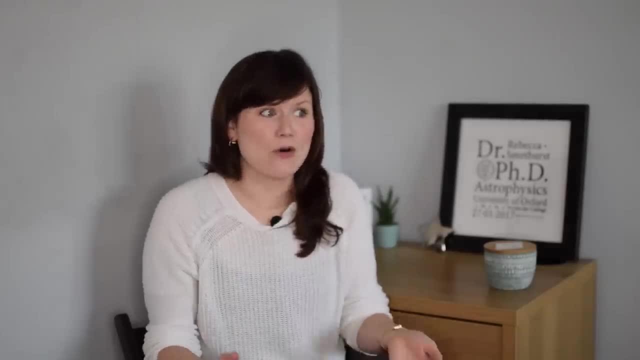 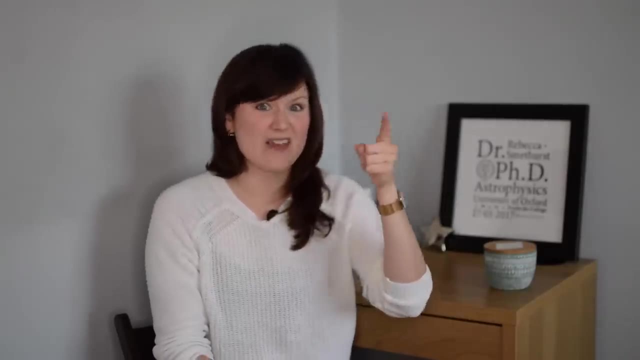 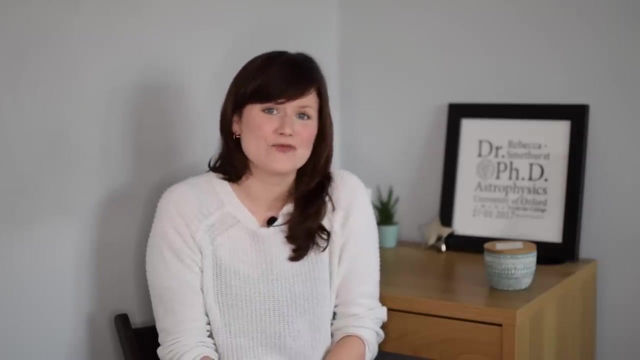 kind of boring and I just really miss talking about space all day and I miss talking about galaxies and stars and black holes, Even though I started in September. by the November I was ringing my masters supervisor again saying I think I've made a terrible mistake and I really want to come back to astrophysics because I've remembered that. yeah, I want to be. 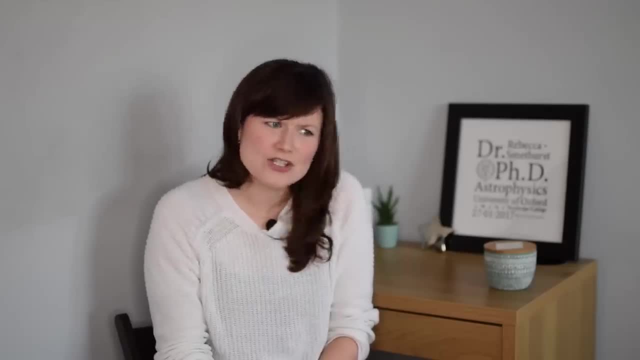 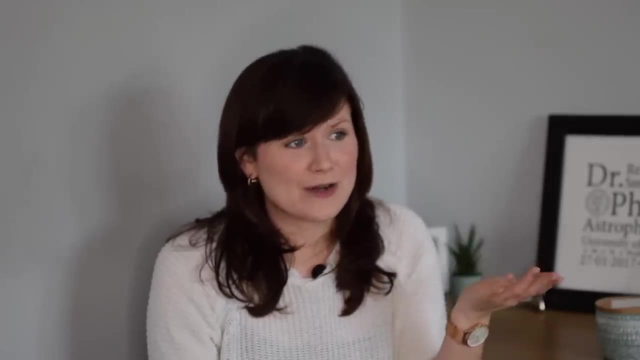 a scientist, I want to think and answer questions that no one knows the answer to. that's what I want to do and what I want my job to be. So it took me a while of figuring out what I actually wanted to do with my life, because, admittedly, that was my fault, because I procrastinated the decision. 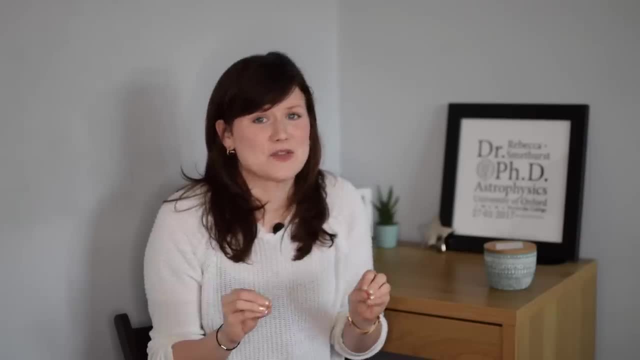 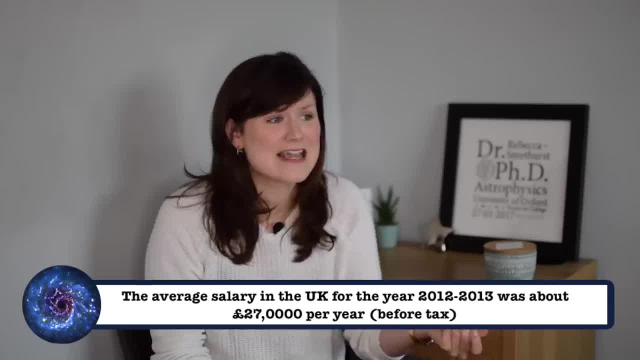 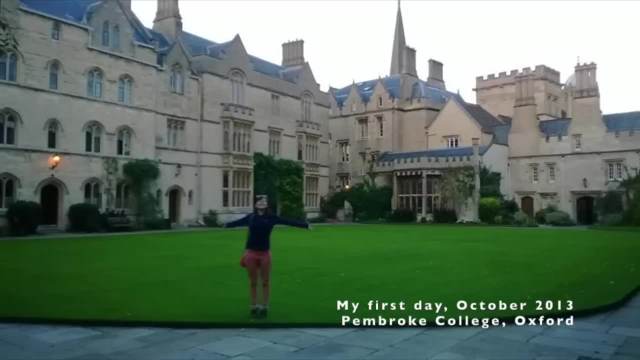 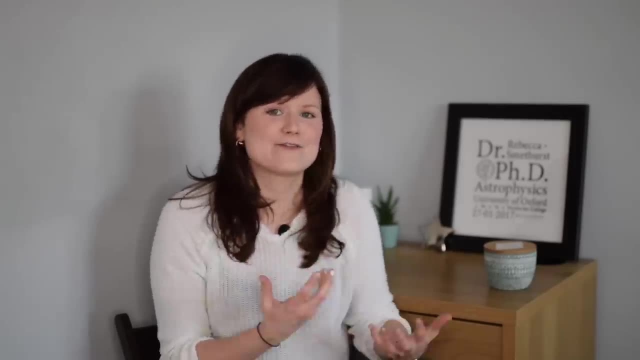 very good job that was paying something like twenty eight thousand pounds a year to go back into education and do a PhD, and that was what I did at 23.. I started a PhD at Oxford researching all about how galaxies change their shape over the lifetime of the universe. 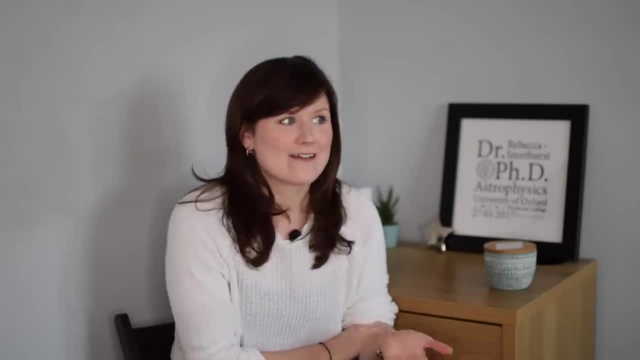 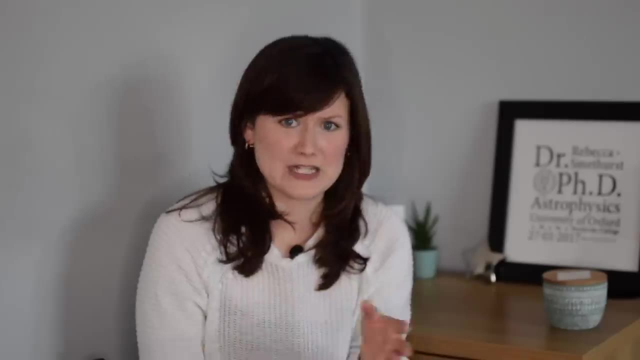 and I had never been happier. I didn't care about that paper. I'd gone from what twenty eight grand a year to being paid a grant of about thirteen thousand pounds a year which was taxed free, didn't have to pay my student loan back, national insurance free, and so it was essentially 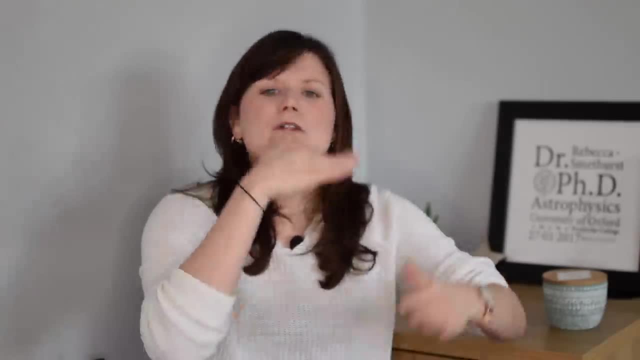 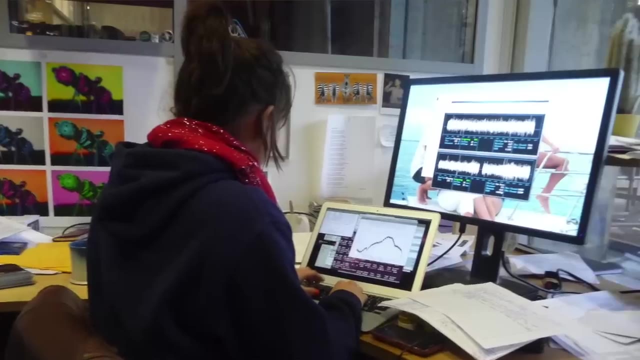 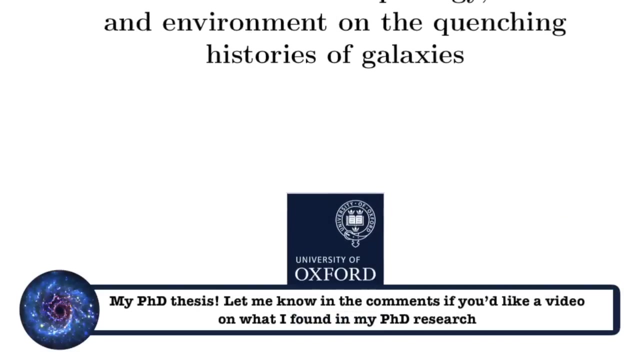 like being paid a wage of about twenty thousand pounds after tax. But I was really happy. I was talking about space again and I was working towards writing my thesis, this huge, big document that essentially outlines all of the independent research that you've done over three years under. 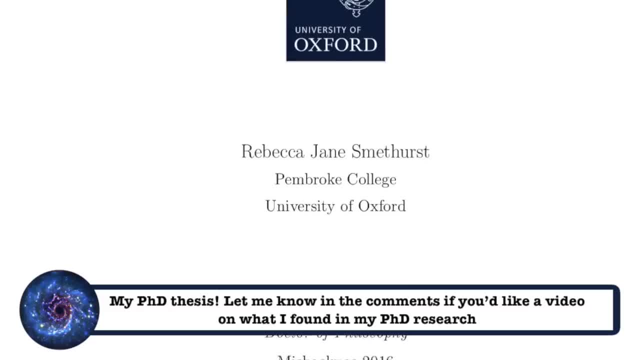 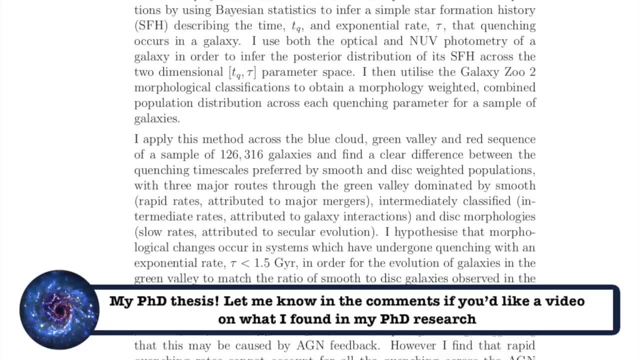 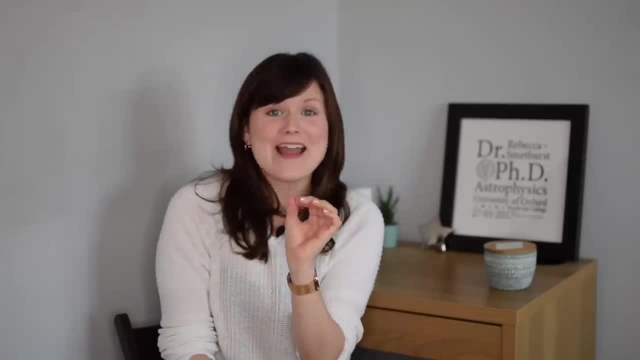 the supervision of your PhD supervisor advisor, And a PhD is there to prove that you are an independent researcher by the end of it, That you can come up with a question that we can ask about the universe or the world that we live in and, most crucially, a feasible way of actually 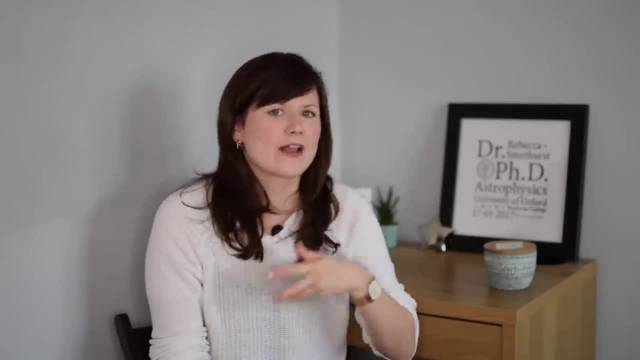 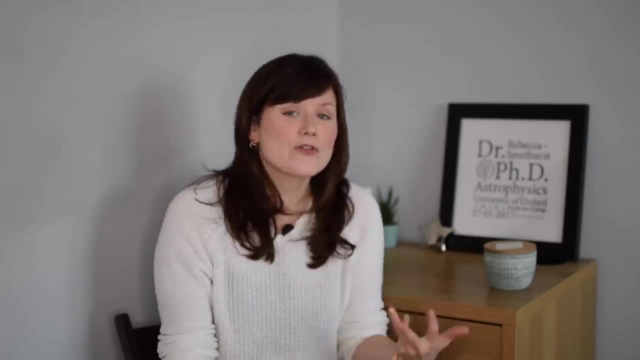 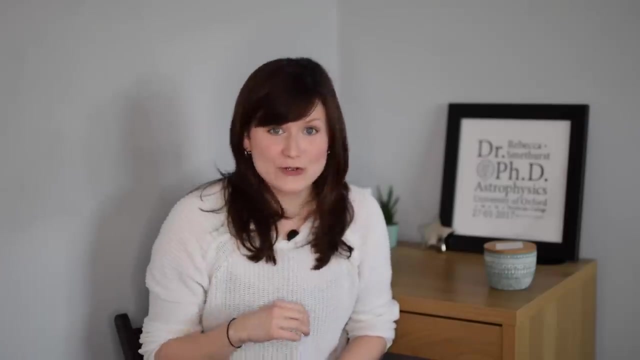 trying to answer that question and then you can report back on it, get your findings published and show to the world that you are someone who is knowledgeable and an expert in that incredibly specific subject that you have focused on during your PhD, During my PhD. 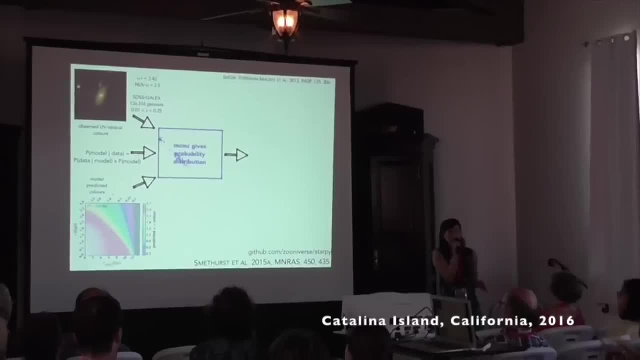 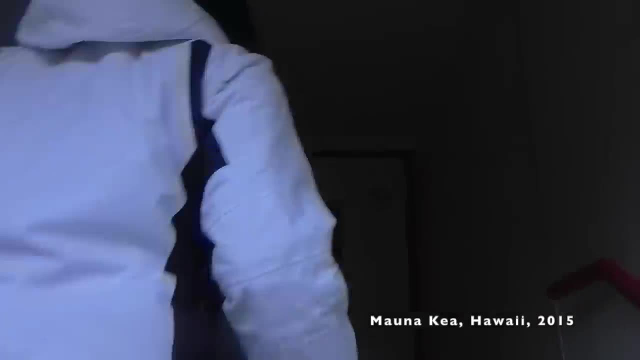 I got to go all around the world on conferences, presenting my results, talking to other researchers. I got to use telescopes in La Palma and in Hawaii as well, which I still can't get over- the fact that they pay you to go to Hawaii Before I could graduate from my PhD, though. 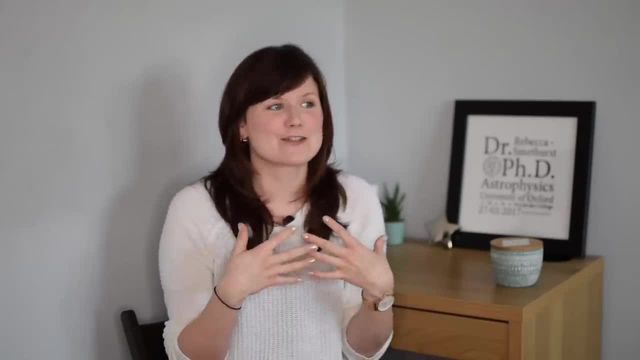 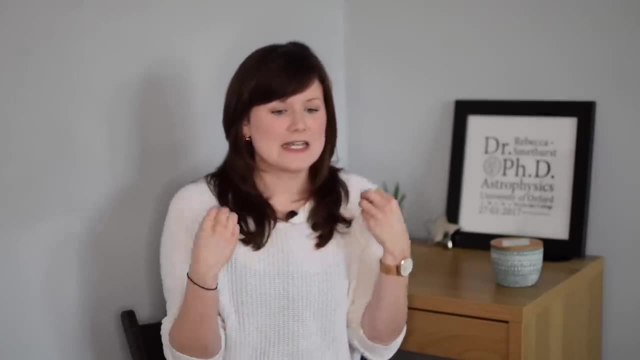 I had to prove that it really was all my work, and so I had to go into a thesis defense exam, what we call a viva. It's essentially an exam where you sit in a room with two other people who are experts in your field. they've read your thesis beforehand, and then they pour over it. 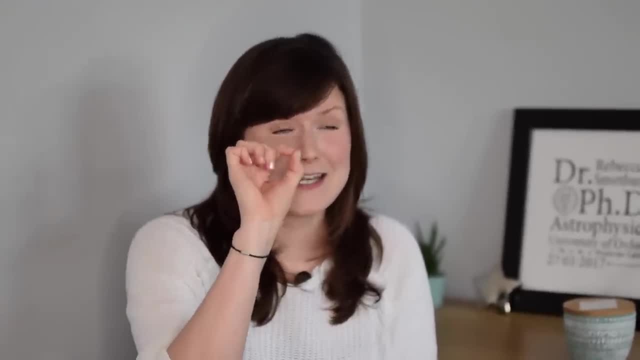 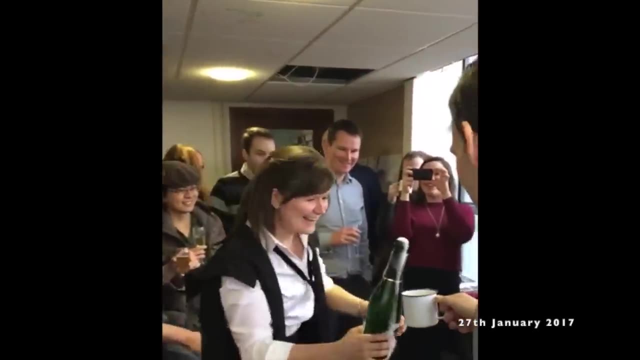 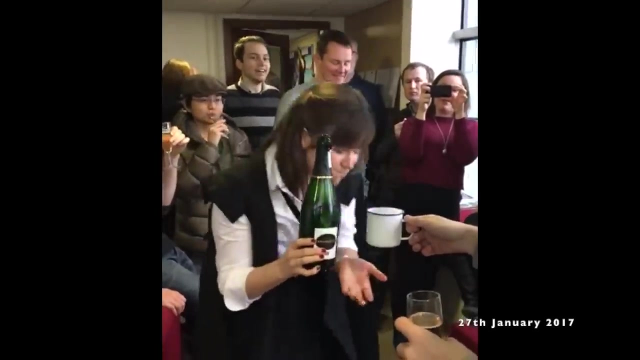 and question you on every specific tiny little detail in there. Thankfully, I passed my viva after a three-hour grilling from my examiners and I've just realized that I'm recording this on the three-year anniversary of passing my viva as well. so kind of all the feels right now. 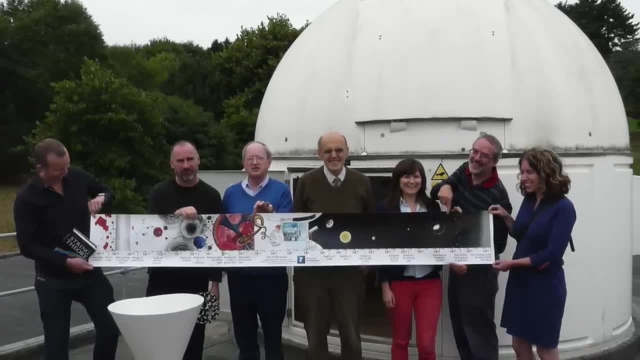 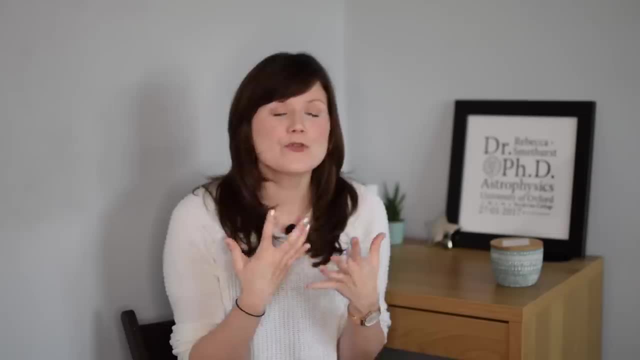 Since then I've had two jobs as an astrophysicist in universities doing research, One at Nottingham for two years and now in Oxford, which I've been there for 18 months- and both of those jobs are what are called research fellowships, So instead of a professor who has specific research, they 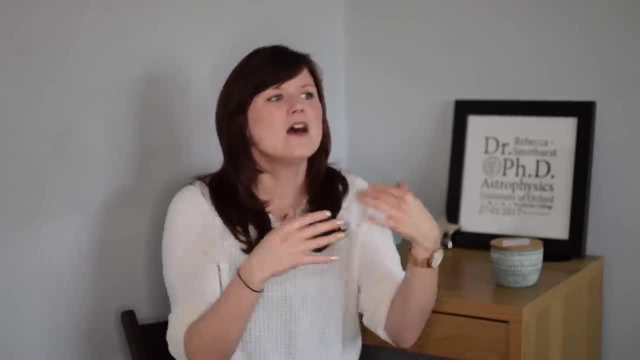 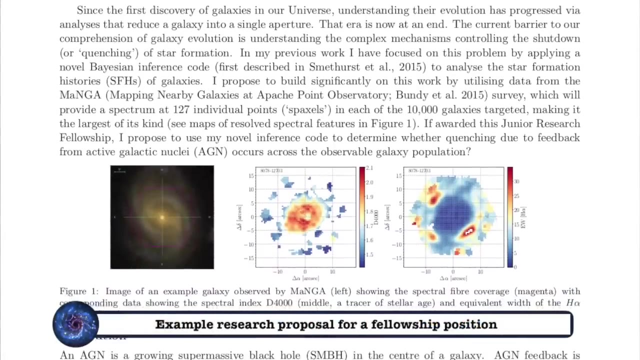 want doing, and so they advertise that job for someone to apply to do it. a fellowship is like: we have this pot of money. tell us what research you would like to do and if we like it, we will pay you to do that research. So at Nottingham I started on a similar salary to what I'd left. 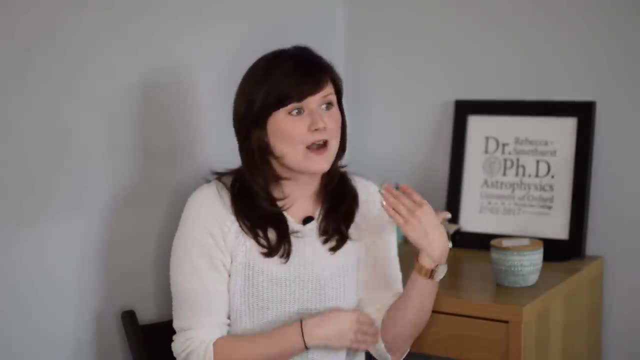 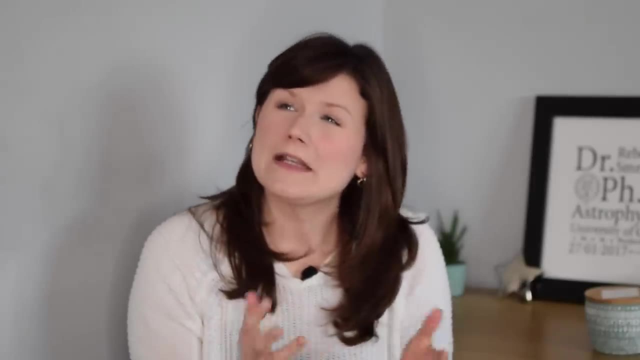 Rolls-Royce at, so I bounced straight back again after my PhD, and then, when I moved to Oxford, my wage increased about 20% more on top of that as well, which means I'm now paying back about 120 quid a month or so on my student loan. That's not much at all. I think every decision I've ever 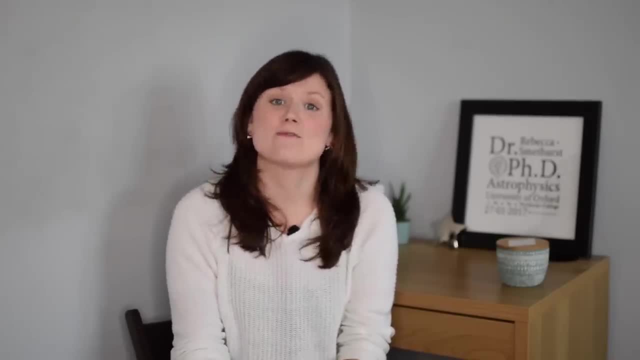 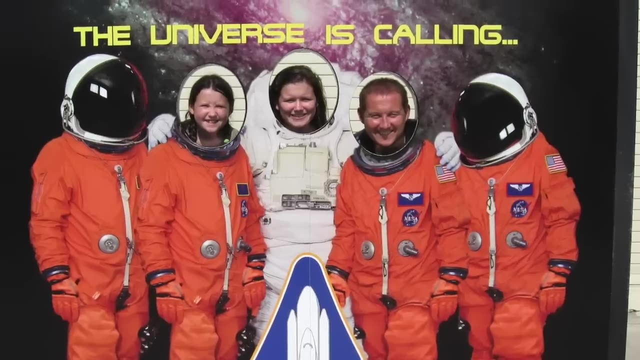 made has always been motivated by a piece of advice my dad gave me when I was younger, which was: do something you love and you'll never work another day again in your life, and that's always resonated with me. So at school, I picked subjects I absolutely loved, because I knew that I would 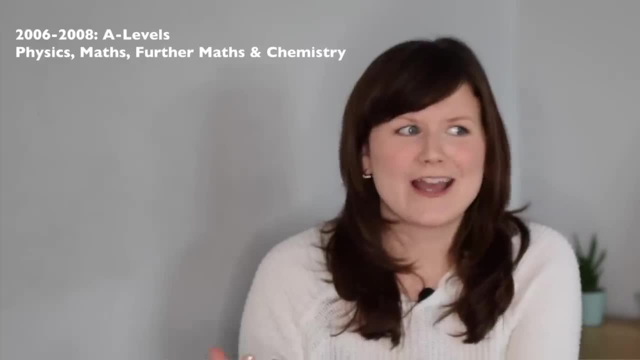 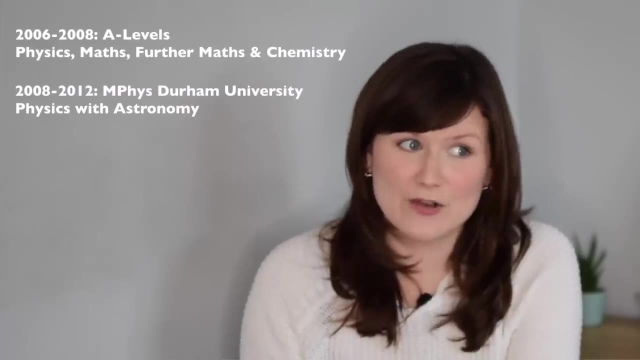 actually want to learn and want to do the work and therefore get good grades. At university, I did a subject I loved because I knew that it would eventually lead to a career that I loved, even if I didn't know what that was at the time. and then I went to do a PhD because I knew that. 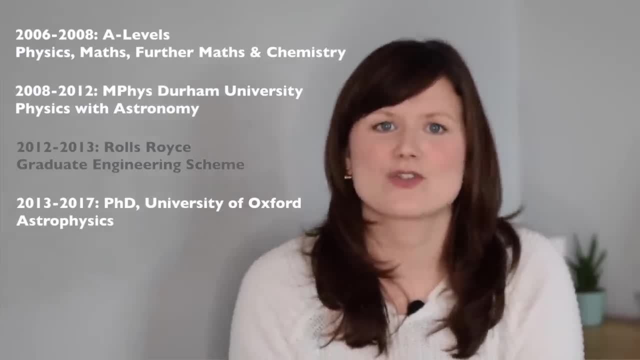 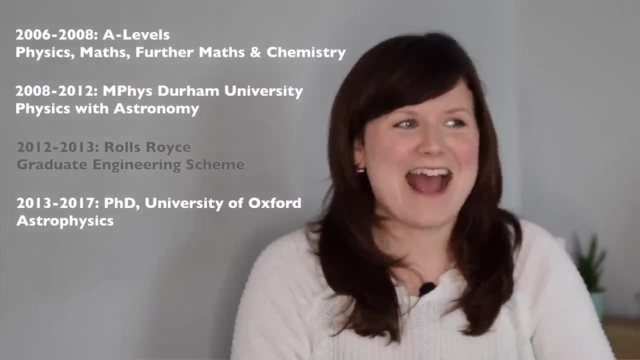 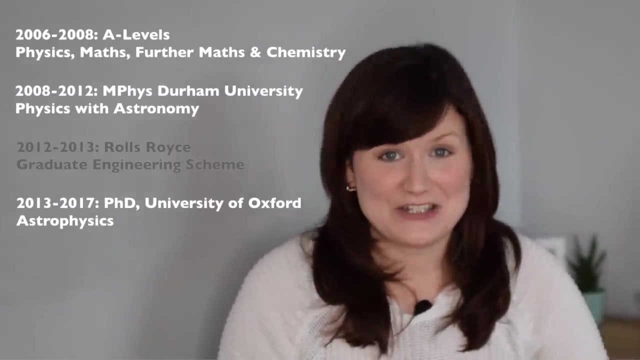 that was the way that I would get to call myself an astrophysicist, a scientist, and I would be able to do what I loved every single day, which was talk about space and answer the questions that we still don't know the answers to, or at least try to do that, because I'm still learning All. 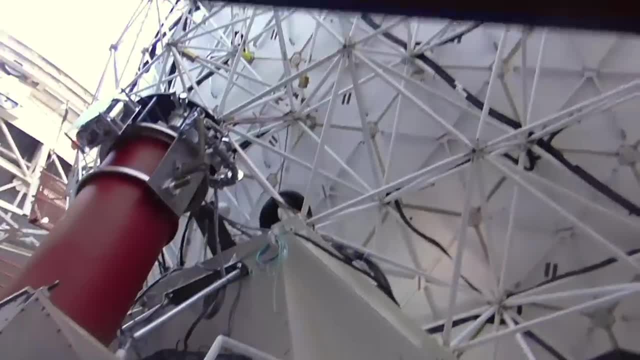 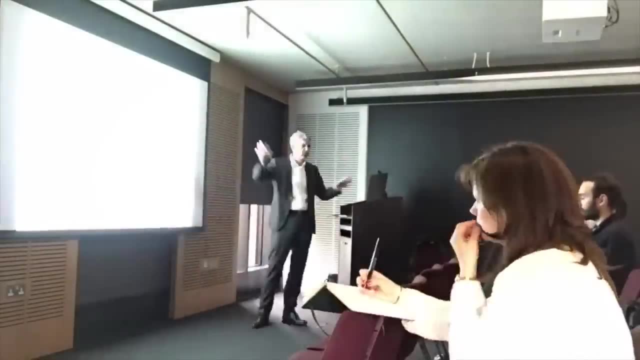 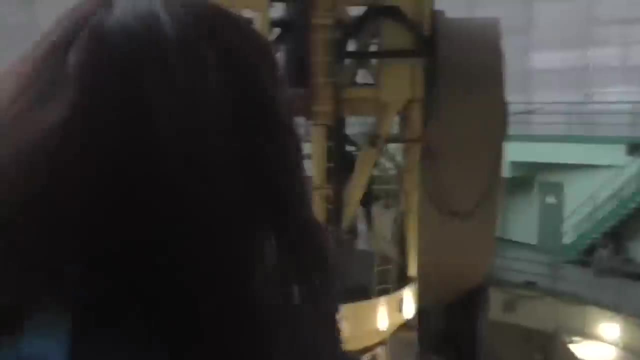 scientists are still learning all the time, whether it's about the universe or a disease or computers, and by getting new people into science we get different viewpoints on problems that haven't been solved for decades and we learn more, and that's always what I've loved to do in. 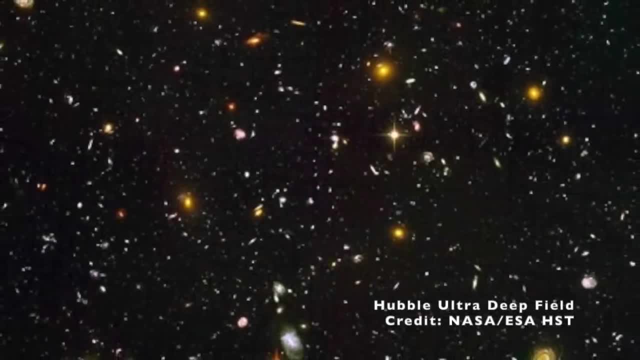 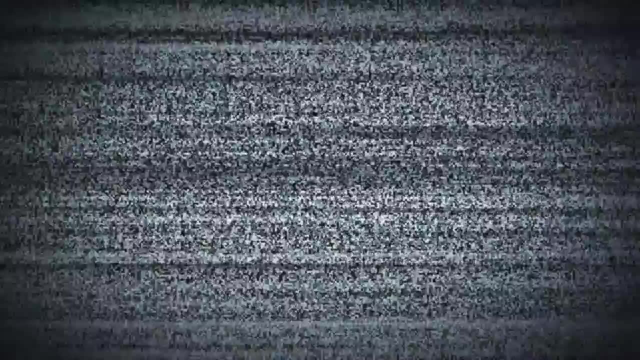 life is to learn and be amazed that we even have the hope that we can do something that we love, The hope of understanding a tiny fragment of what the universe has to offer. Dance, monkey, dance, monkey, dance monkey, oh, oh, oh, oh, oh oh. 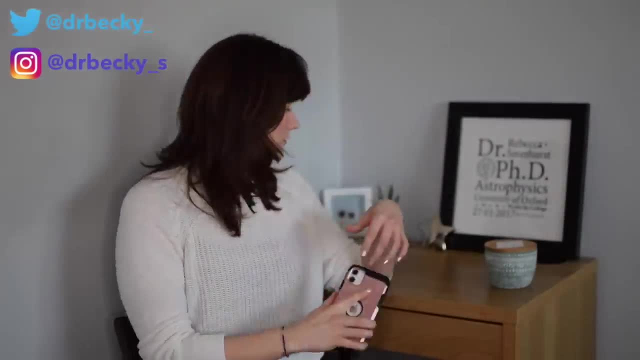 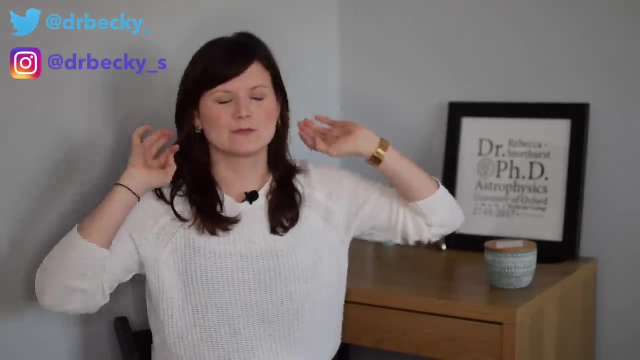 Oh, tangled in my wire. I'm thinking about this new angle. I don't know about it. I don't know how. I feel We've rearranged the room for guests and now I'm this way and you're there rather than there, and I'm like